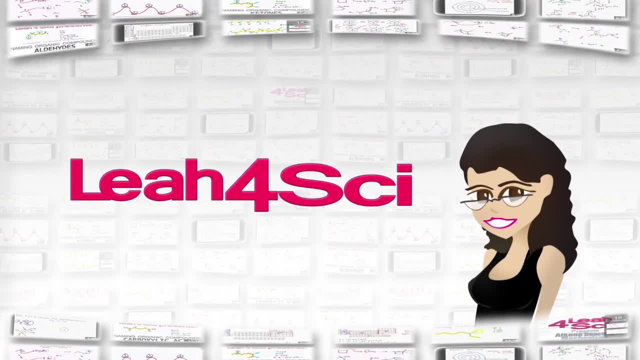 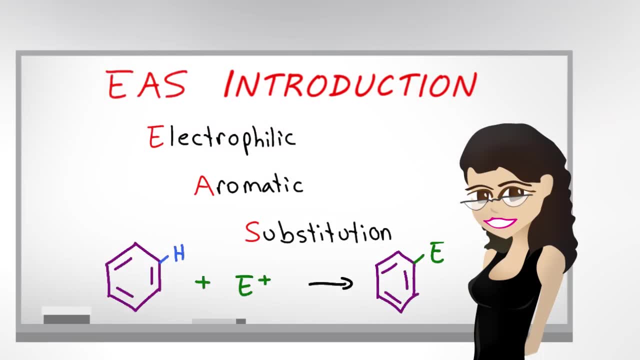 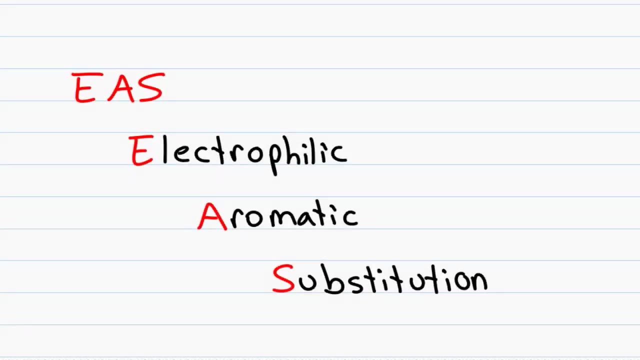 Leah here from leah4scicom, where you can find hundreds of organic chemistry tutorial videos or go cheat sheet study tips and more, and in this video I will introduce the topic of EAS, or electrophilic aromatic substitution. The bad news is, many students find this topic 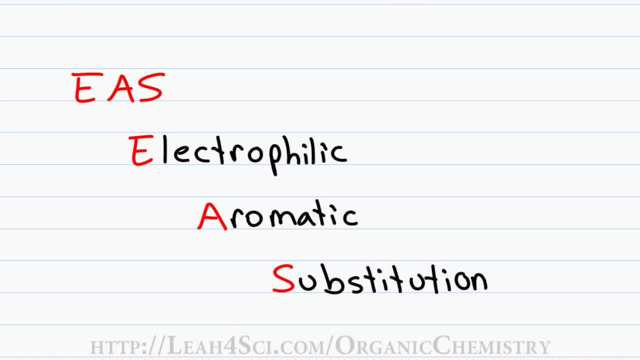 difficult. but the good news is this is actually an easy and fun topic if you understand what's going on, and my goal with this video series is to make sure that you know exactly how to proceed with reactions. But first we have to breakdown EAS to understand what's going. 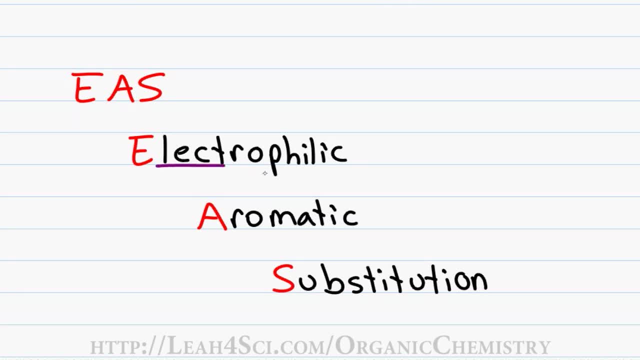 on. Electrophilic comes from the word electro, meaning electron, philic, or phile meaning loving. An electrophile is something that is electron loving, Since opposites attract, something that is electron loving must be positive or partially positive, and so we know. 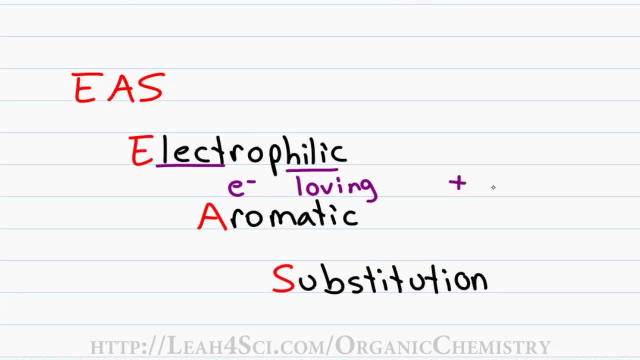 this reaction is going to take place using molecules that are positive or partially positive. aromatic comes from aromaticity, which means a molecule that is cyclic, planar, conjugated and obeys Huckel's rule. Most of these reactions will take place with benzene, but you'll also. 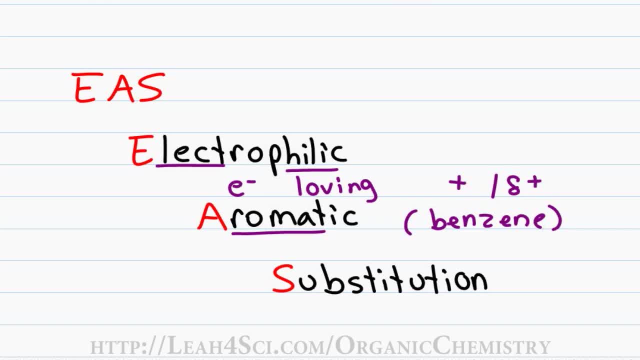 see some other related compounds. And finally, we have substitution, which means we replace one group with another. In this case, we're going to replace a hydrogen with a group that's adding to the ring. Let's have a quick overview. The EAS reaction typically starts out when. 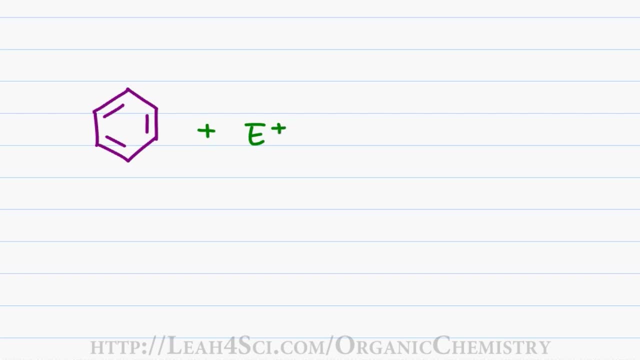 a benzene reacts with a superelectrophile, which we'll explain shortly, to yield a product that has the electrophile attached to the benzene ring. This appears to be addition, but it's really a substitution reaction because, don't forget, we used to have a hydrogen here. 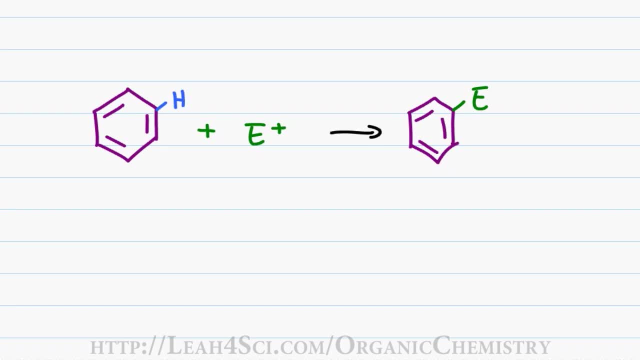 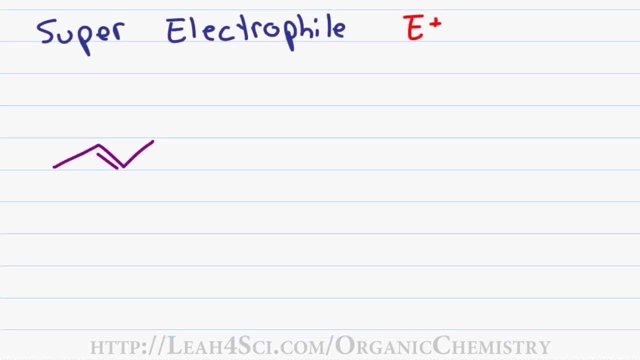 and when that electrophile attaches to benzene, the hydrogen has to be removed and this is something we'll look at in the actual mechanism. I mentioned that this reaction requires a superelectrophile and let's see why by reviewing an alkene addition reaction, Say, I have two. 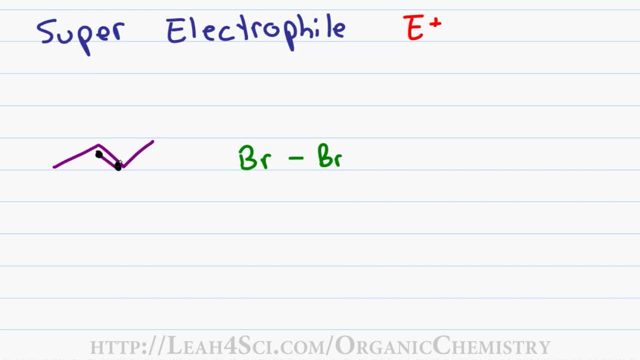 butene, The nucleophilic pi electrons will reach out for bromine, bromine attacks back and the second bromine breaks off. I have a bridged intermediate and so the negative bromine comes and attacks from the opposite side, breaking the bridge and giving me the final product. 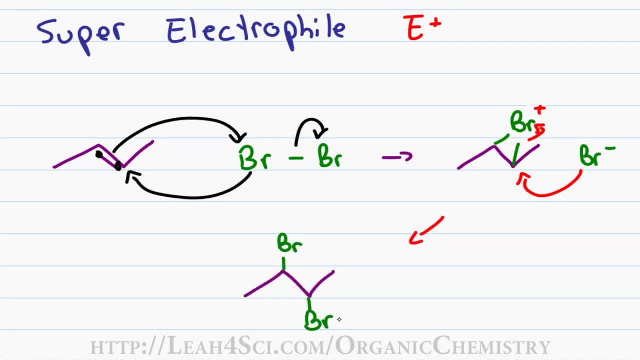 an anti-vicinal dihalide. If you're not comfortable with this reaction, go back to my alkene reaction video series, where I go through it in detail. But what I want to show you here is that pi electrons are very nucleophilic and will attack. 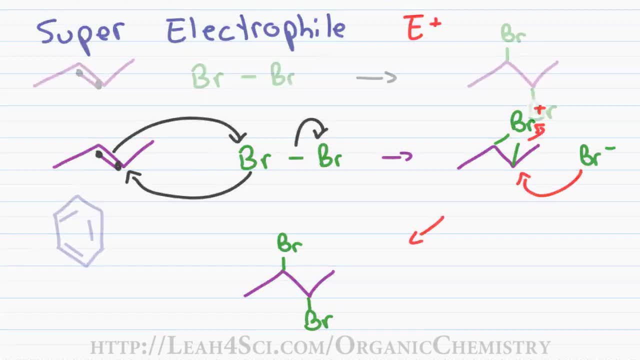 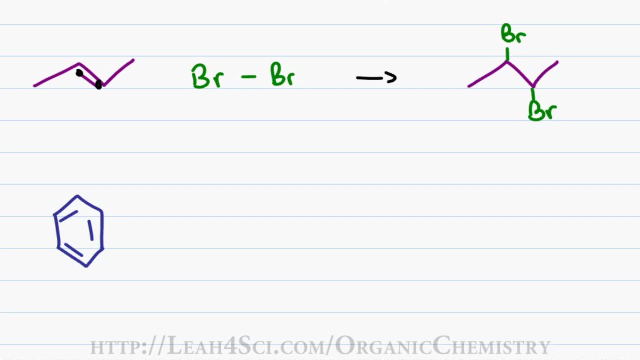 And so it's only natural to think that, if we can add something to an alkene, we should be able to carry out the same exact reaction with benzene, since benzene has three pi bonds, In fact, shouldn't we have triple the product? But in reality, if you try adding bromine, 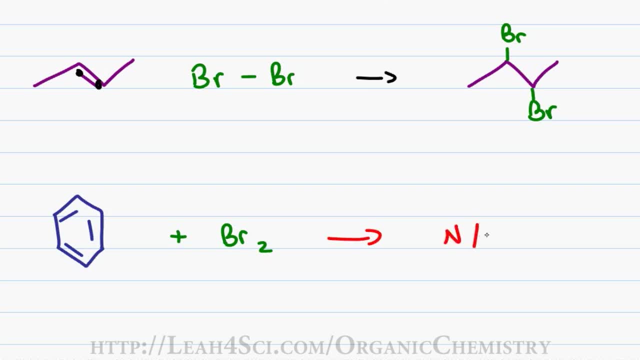 to benzene using the same reaction conditions, you're going to get absolutely no reaction. Why? Because the pi bonds and benzene are a lot more stable than an alkene. In reality, In reactions we follow the rules of happy, stable, unreactive, unhappy, unstable, very. 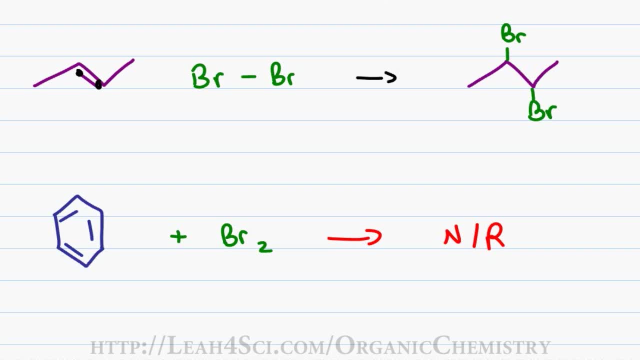 reactive. The only reason a molecule will react is if the next step or the outcome will make it more stable than the starting molecule. But with benzene, if you were to break open the ring for an addition reaction, you're sacrificing the aromaticity or sacrificing the stability, and it's not worth it. 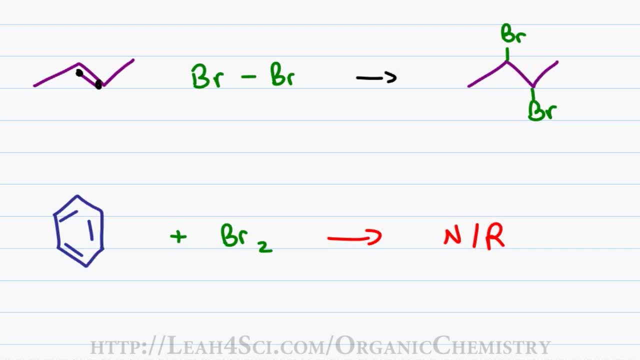 Since benzene will not reach out to attack a standard electrophile, we need something that is so positive and so unstable that benzene has no choice to attack, and this is the idea of the super electrophile. If you compare your EAS reactions to your alkene reactions, you'll notice that the super 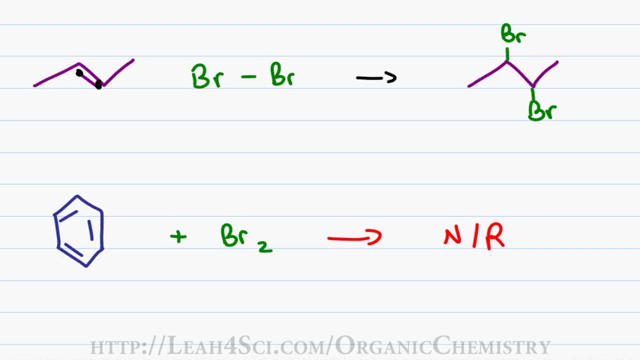 electrophiles are so much more positive and so much less stable as compared to your standard alkene electrophiles. Now that you have an idea of what goes on in EAS and what to expect, join me for the remainder of this series, where I take you through the mechanism for electrophilic aromaticity. 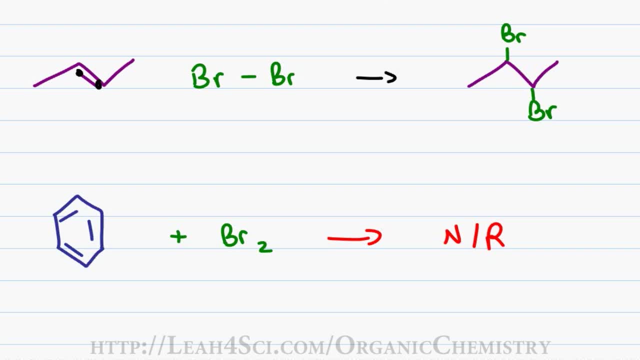 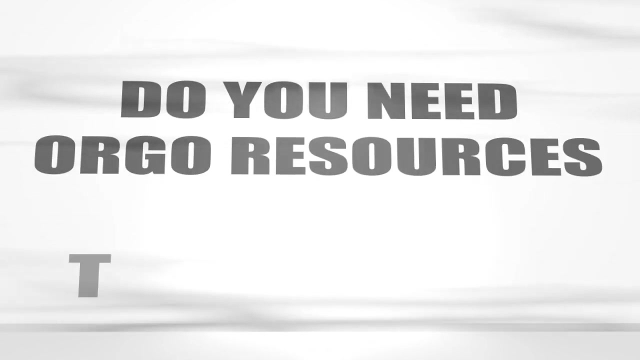 Thank you so much for watching and I'll see you in the next video. Bye. Subtitles- by the Amaraorg community. Are you struggling with organic chemistry? Are you looking for resources and information to guide you through the course and help you succeed?